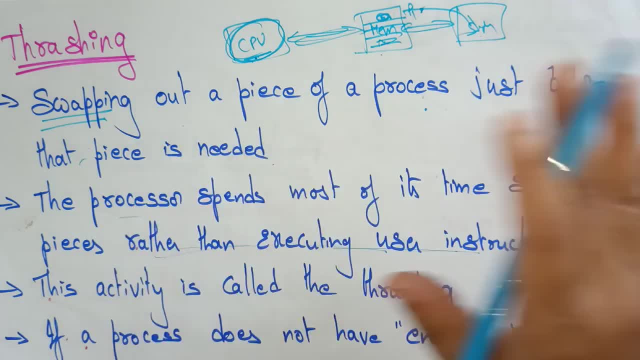 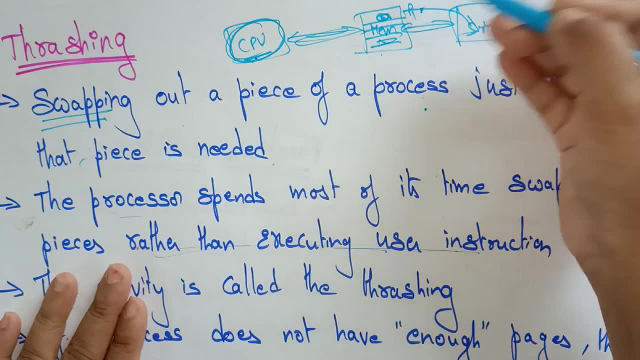 So again it is going to secondary memory and getting the data. So this lot of here every What exactly the CPU is doing here? Here the CPU spends most of its time swapping pieces, taking the pieces and again deleted. taking the pieces, again delete them. 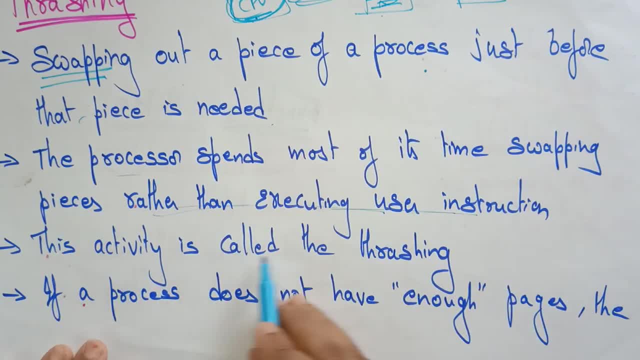 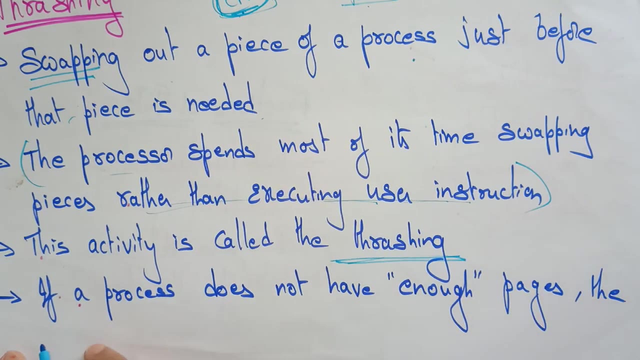 rather than executing the user instructions. so this activity is called thrashing. so what exactly the thrashing means? whenever the processor is not doing anything, still it spends its time on swapping rather than executing the user instruction. this activity is called a thrashing. it is a process. 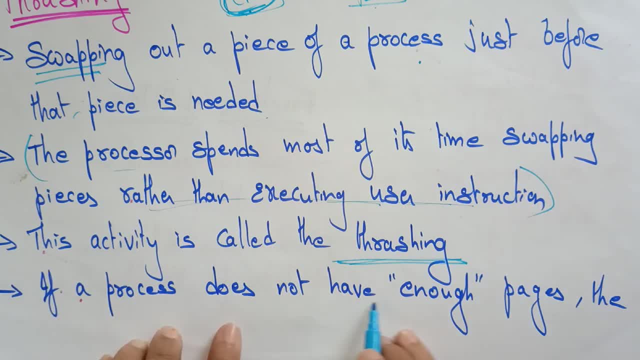 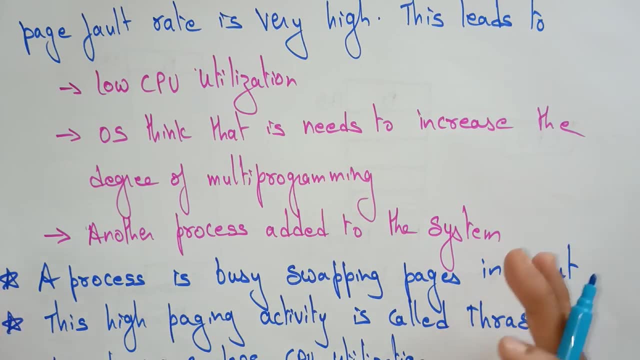 done does. uh, sorry, if a process does not have enough pages, the page fault rate is very high. the page fault rate is very high means every time is going to the secondary memory and getting the page and again if that page. suppose the cpu wants some page in the main memory if that page is not, 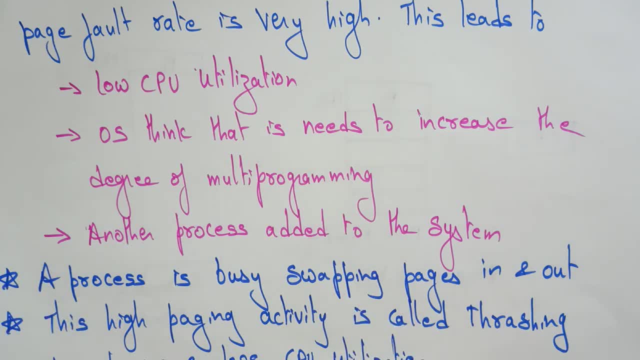 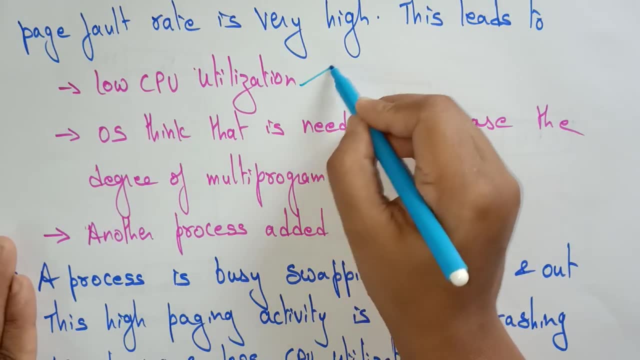 present, then the page fault is occurred. so again it is going to the secondary memory and getting the page. so here the page fault rate is very high. so if the page fault rate is very high then it leads to low cpu utilization means here cpu is still doing the work on swapping rather than 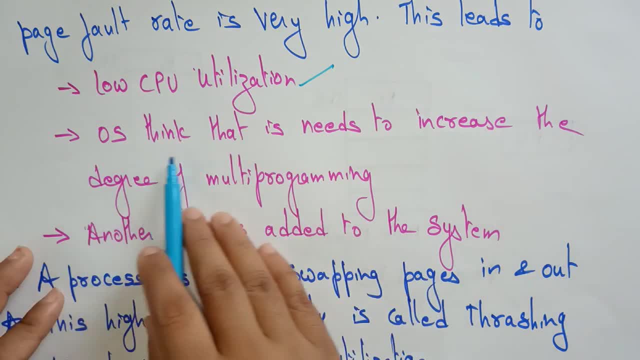 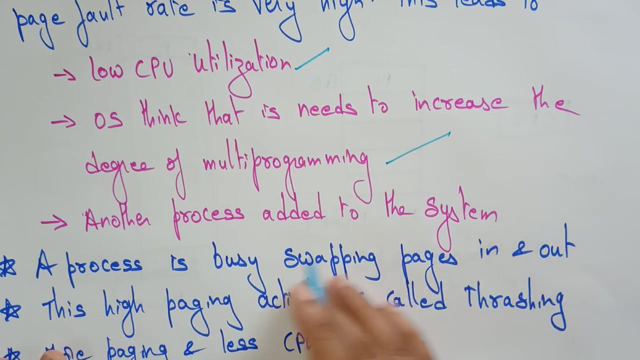 executing. so cpu utilization becomes low. operating system think that it needs to increase the degree of multi-programming. so here the operating system is also thinking in another way. it thought that, okay, we need to increase the degree of multi-programming because cpu utilization becomes slow. another process adds: 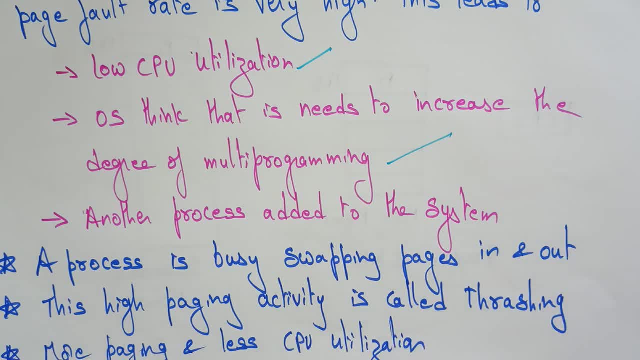 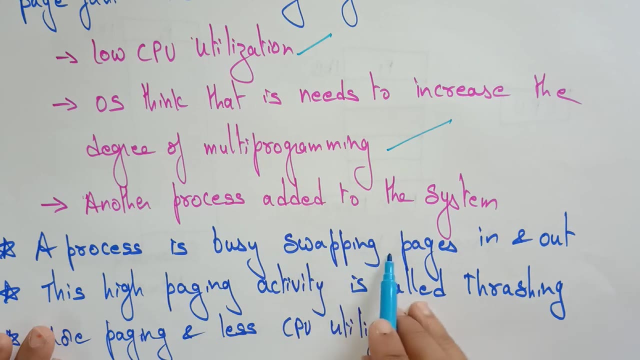 to the system. here we are not completed. one process but another process is ready to add to the system. so this is uh. because of this, page falls. these are all the problems that this uh system is going to to lead. this leads to a process is busy swapping page in and out. the high paging activity is called. 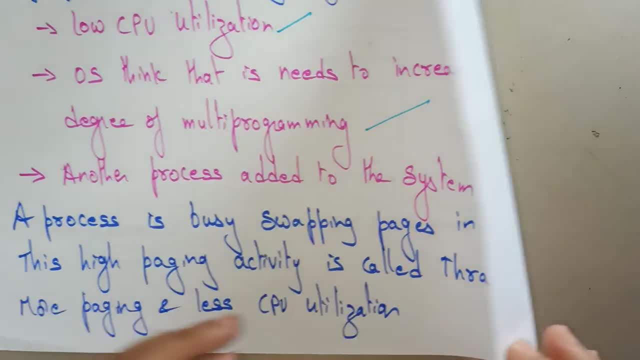 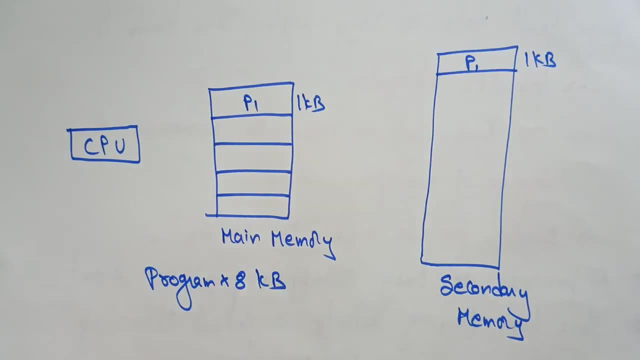 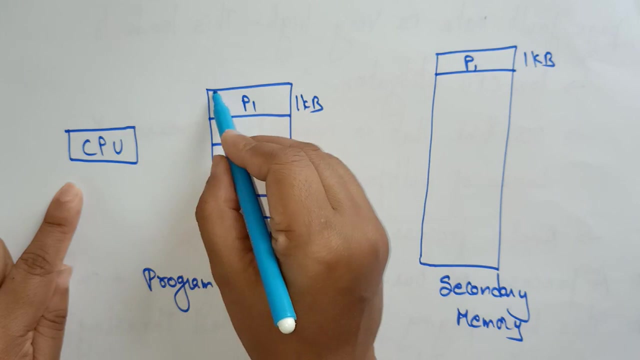 thrashing: more paging and less cpu utilization. okay, so what exactly? the more paging and less cpu utilization. let me explain you with this example. okay, so here my cpu is there. i'm taking the main memory. this is my main memory, a main memory consisting of each size of the block size. 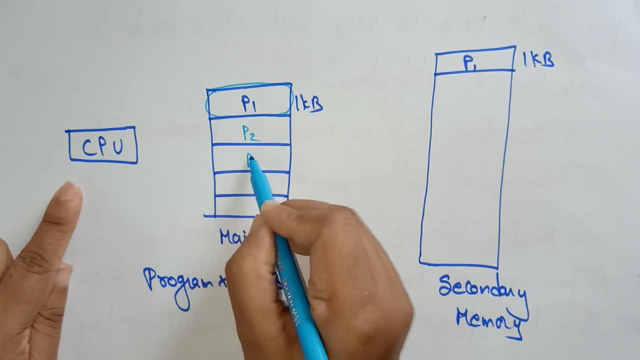 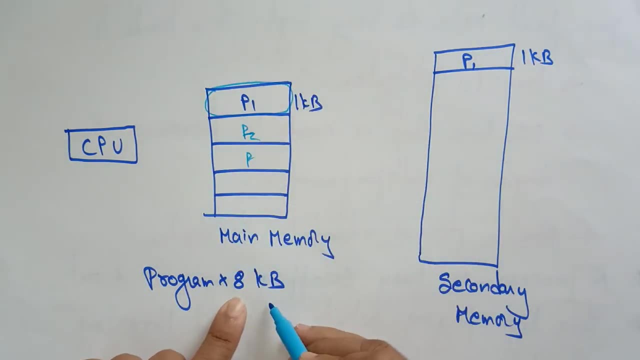 is 1 kb. so here i'm inserting page 1 page. let's take page 1, page 2 page that i want to insert in the main memory, okay, so my main memory size is 8 kilobytes. the size of my main memory is 8 kilobytes. 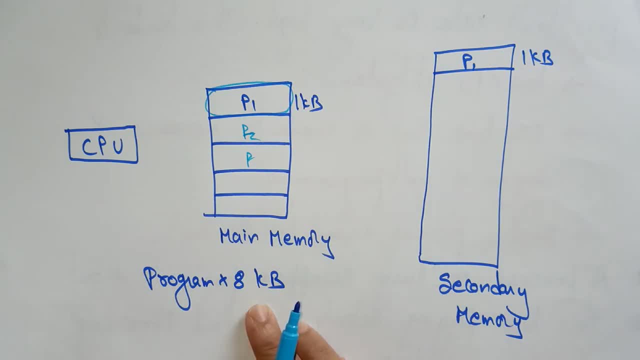 until 8 kilobytes only it can store the data. okay, so now my cpu wants to execute, p1 wants p1 processor, so it gets the data from cpu. okay and no problem, because it is present in the p1. now again. uh, the p2 will be taken. 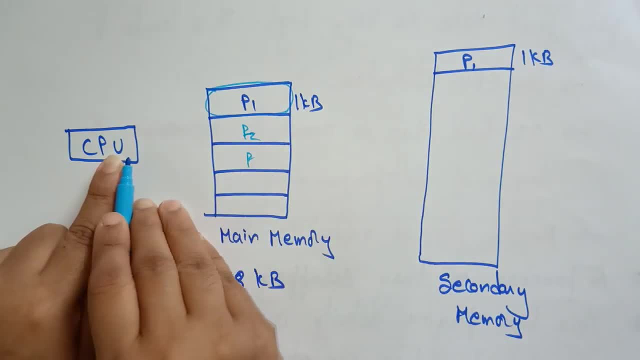 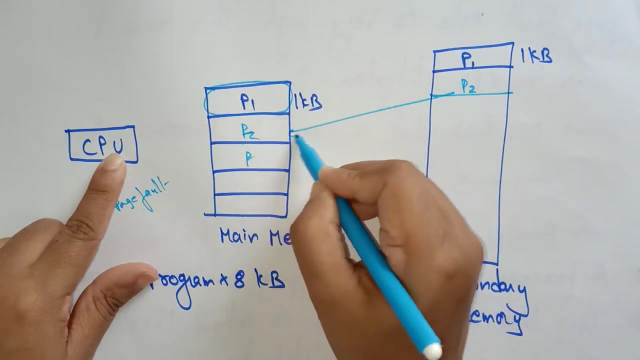 from the uh. now the cpu wants uh process p2, but p2 is not in the main memory. then the page fault is occurred. okay, page fault is occurred. whenever the page fault is occurred, the cpu sends the controller to the secondary memory and get that p2 and place it on main memory. now the cpu will. 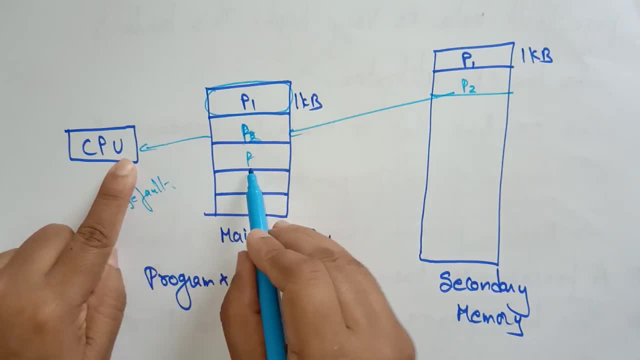 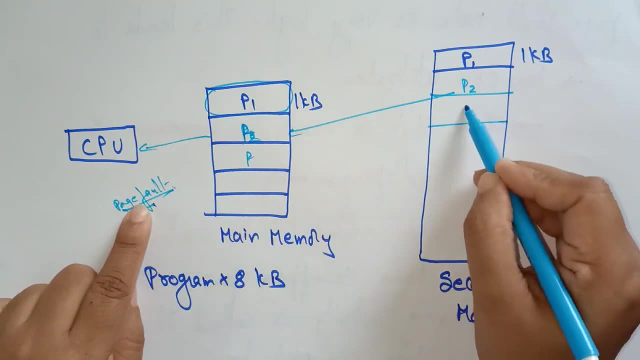 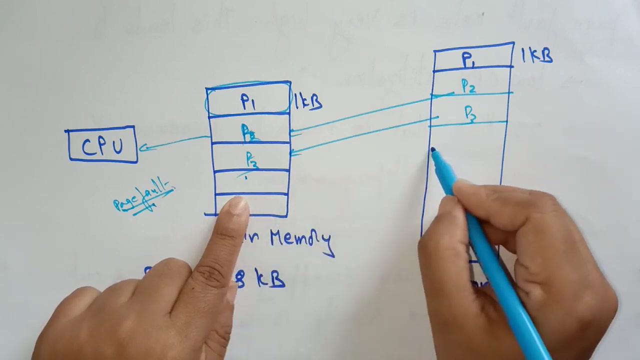 take that page again. the processor wants the page p3. okay, it is not in the main memory. so the again the page fault is occurred. so the controller goes to the secondary memory and take that page and place in the main memory. so like that, it wants the p4, but p4 is not there. so then again the page fault is occurred. so see here: 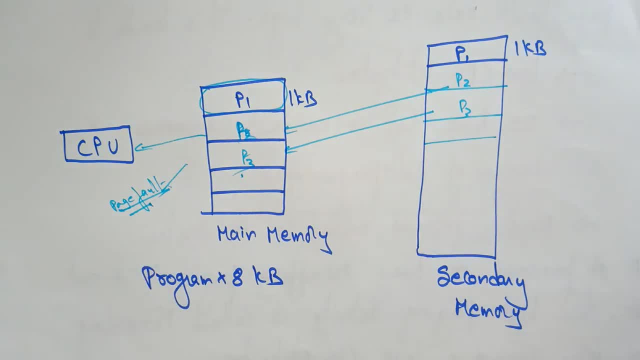 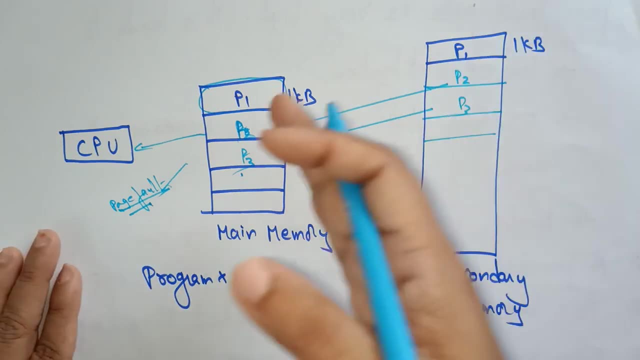 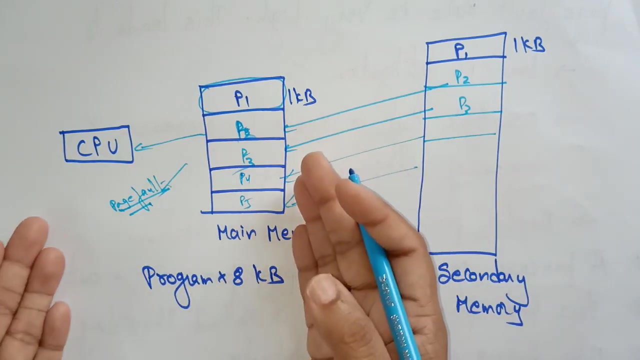 the page fault is increasing. okay, so here, uh, it is, the fault is increasing the cpu, still utilizing the uh time to get the data from secondary memory and place it in the main memory. so it is doing the same work here. okay, just doing getting the data and placing in the main memory. 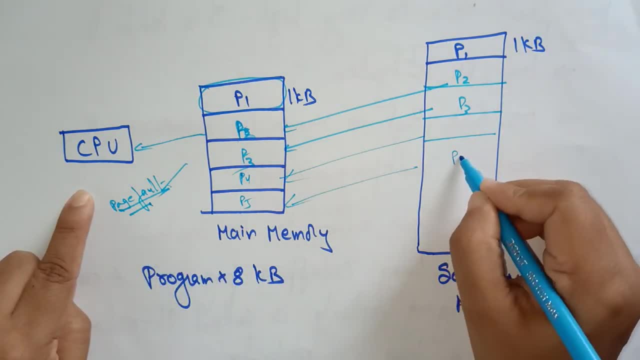 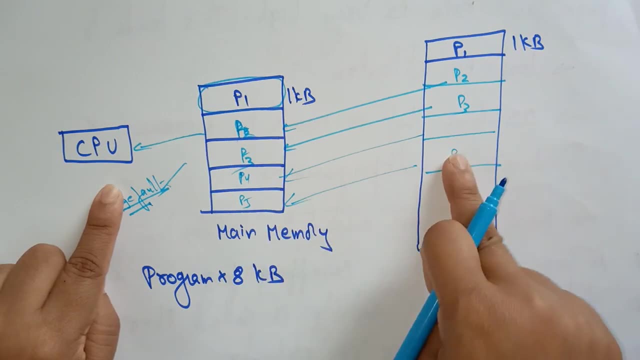 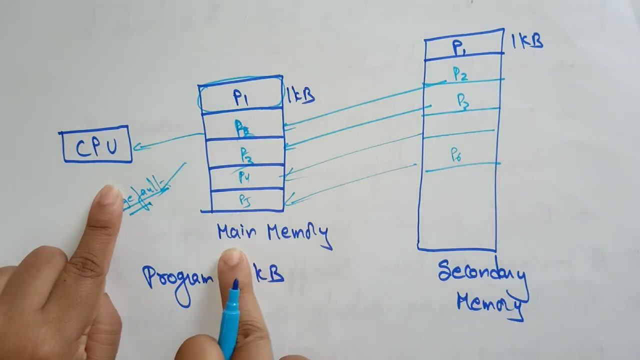 okay. so now my cpu wants a page six. it wants a page sticks to execute, but page six is not in the main memory. okay, it wants to gets from the main, uh, secondary memory. but here my main memory is full with pages P1, P2, P3, P4, P5. already it is filled with the pages now where i have to place. 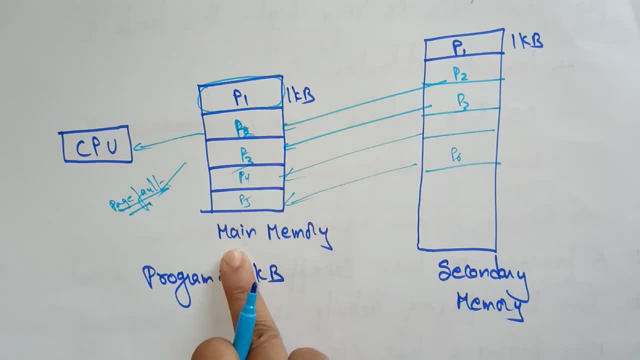 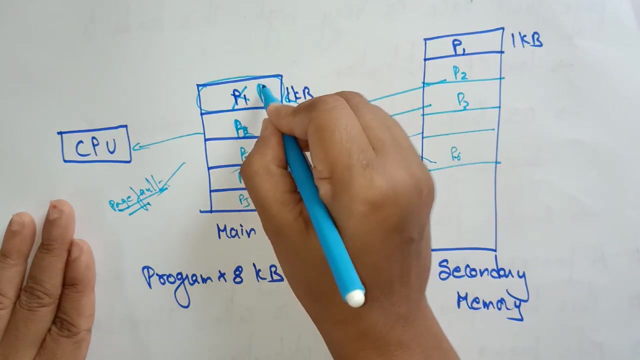 my page. okay, but the cpu wants p6. until that the processor will not execute the user instruction it it wants the page six, secondary memory. Okay, it is very compulsory. So it takes that page 6 and delete the page 1 and occupies page 6 here. Okay, now CPU wants to execute the instruction, But before it executing, 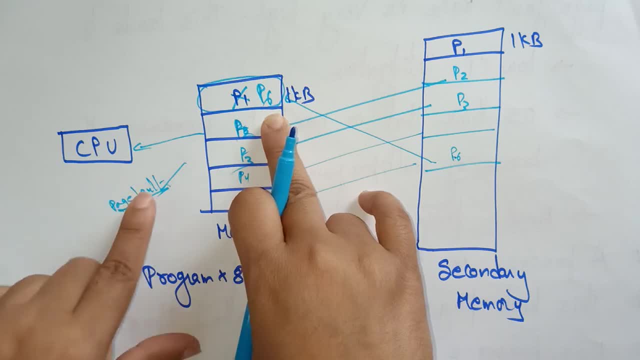 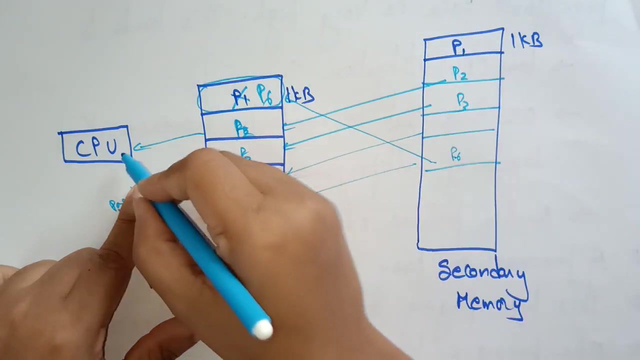 the instruction it requires before executing the P6, it again requires P1 because P1 is having some information that user variables are there that it wants to use. So again the page fault is occur. So then it again go to the P1 rather than executing the current instruction. it again 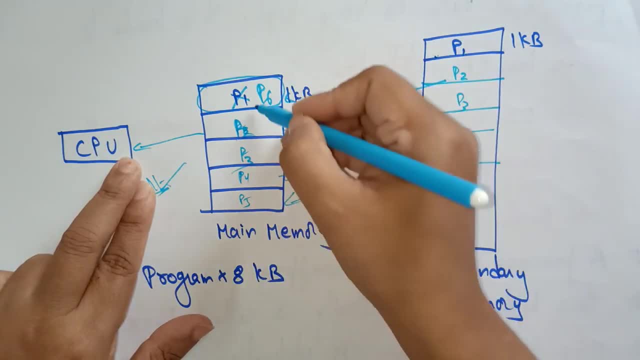 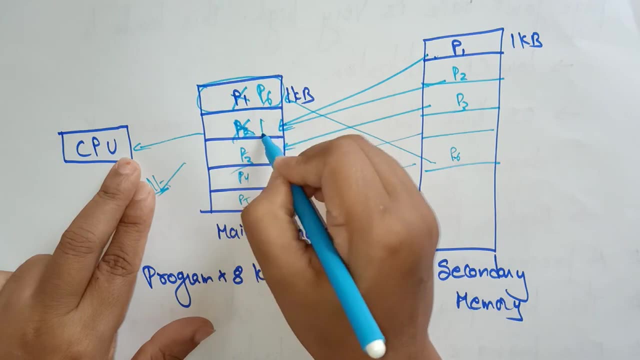 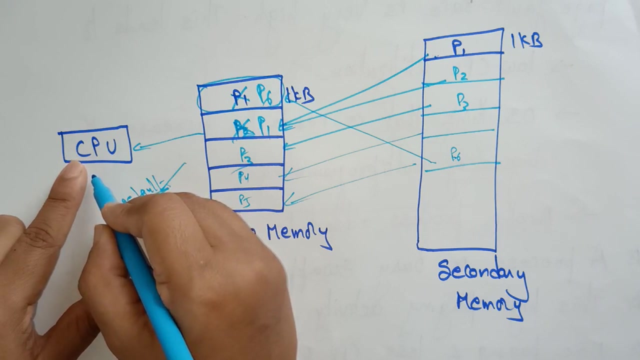 go to the P1, the controller goes to the P1 and gets Then where I need to be insert. It's already my main memory is filled. So again, place that P1 in the second place and deleting the P1.. Okay, now CPU is checking. Let's execute the instruction. But again CPU wants P2 instruction. 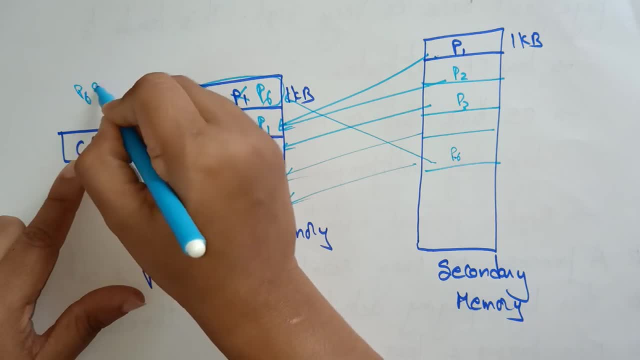 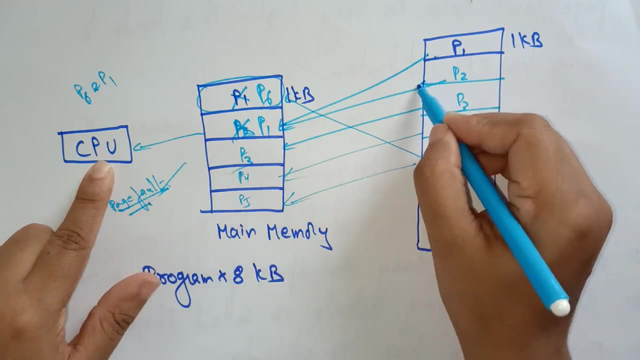 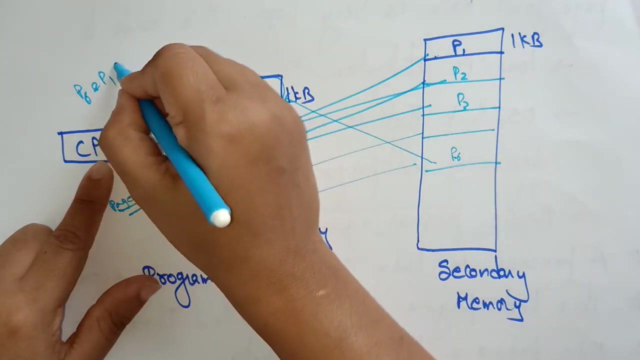 Without P2 instruction, the P6 and P1 will not execute. It wants the P1 instruction, P2 instruction also. So the page fault occurred Again. go to the P2 and get that and the main memory is full. So delete the P3 and P2.. Okay, so again, if you want. 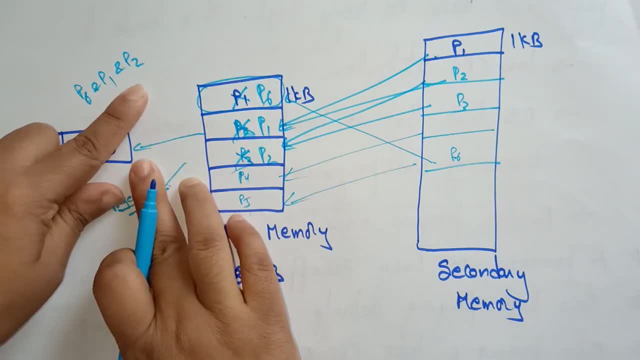 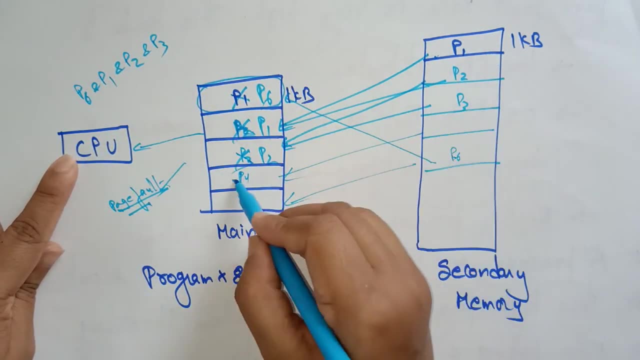 now it has to be execute P6, P1 and P2.. But before executing all these three instructions, it wants again P3 instruction also. Okay, so again, get and place. So like that it is everything. this completely is called swapping. 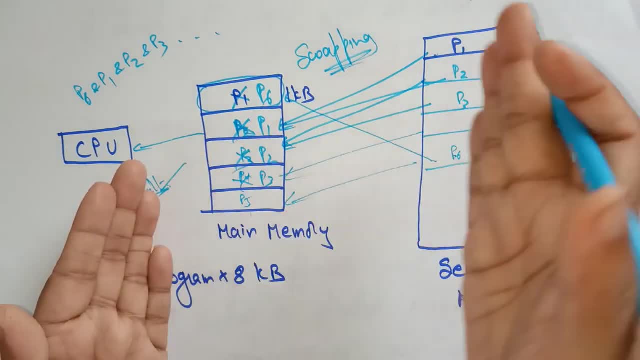 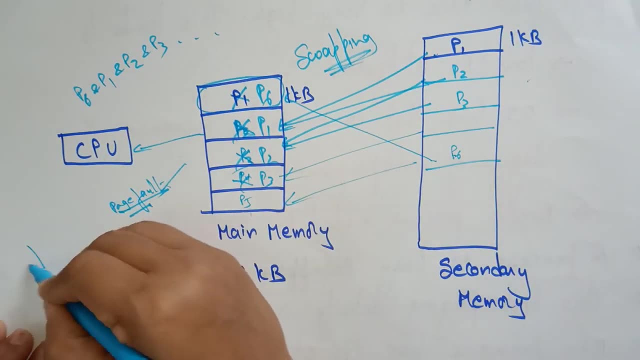 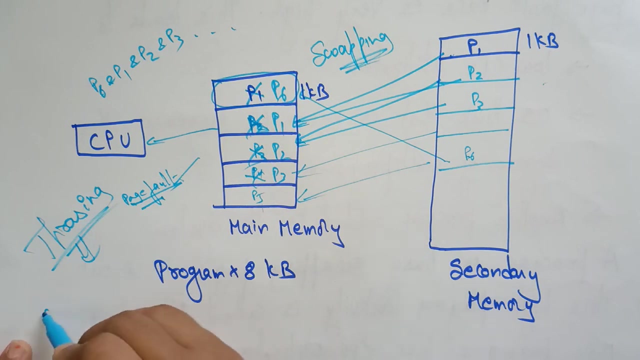 Okay, it is just attacking the pages and removing and updating, removing everything it is doing. that, So this complete process, you call it as a thrashing. So in thrashing what CPU is doing, the thrashing means CPU is utilizing its complete time in 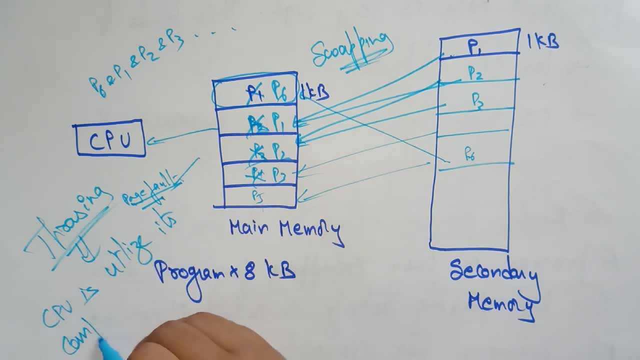 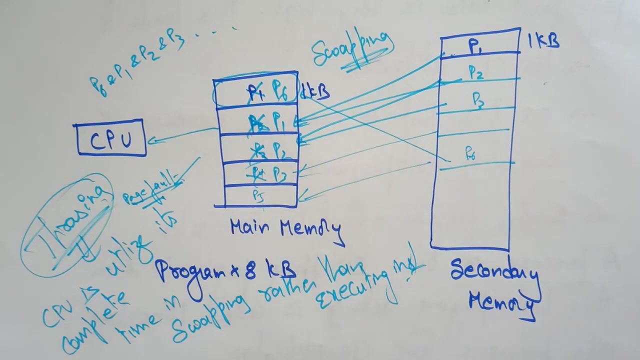 utilize its complete time, complete time in swapping rather than executing the instruction, rather than executing the instruction. so this technique, you call it as a thrashing. i hope, guys, you understand what exactly the thrashing is. here the cpu is spending its complete time in getting the data and doing and getting and. 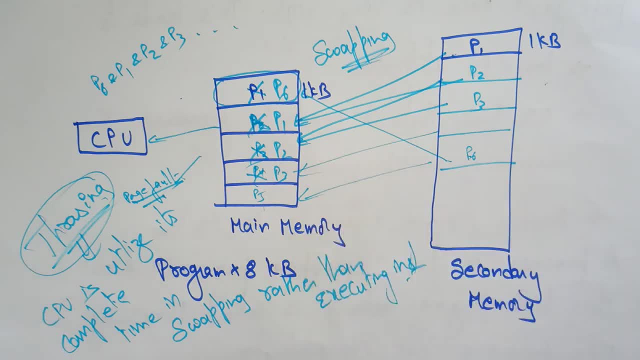 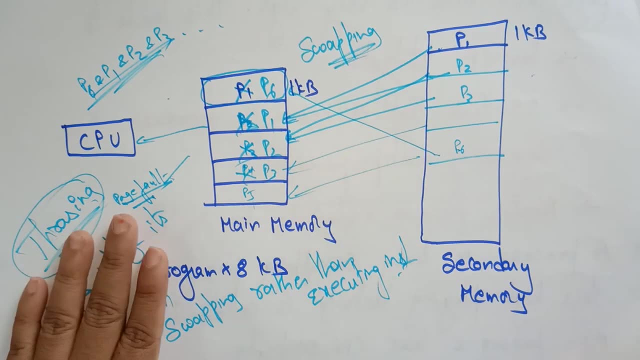 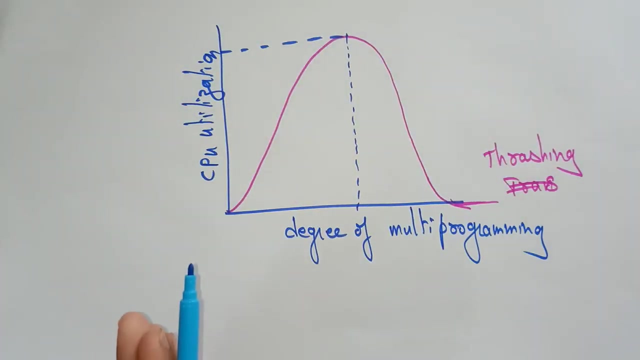 deleting, getting everything. it's completely using its time in swapping. rather than executing the current instruction, it is doing its operation. so here this technique, you call it as a thrashing. so here the page fault rate is very high and the cpu utilization becoming low and the operating 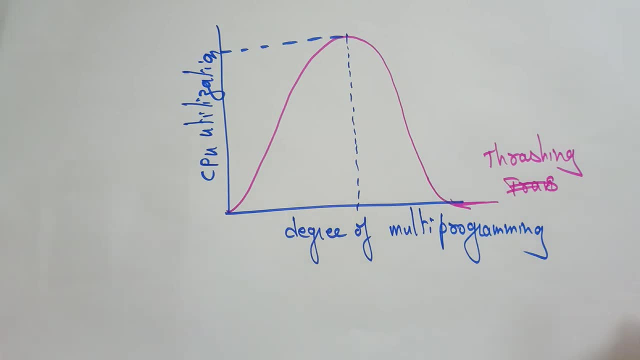 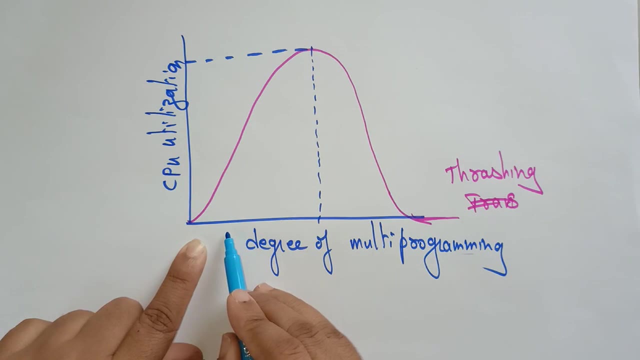 system think that it needs to increase the degree of multi-programming. so here you can clearly understand with the help of this graph here: this is the degree of multi-programming. here operating system thinks that it needs to increase the degree of multi-programming. the degree of multi-programming in: